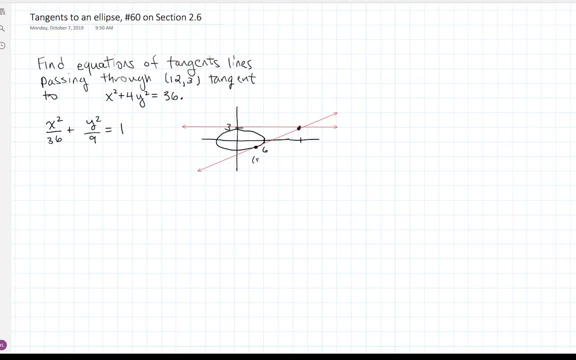 line hits the ellipse And I'll make a couple observations about that point, together with the- you know- information about the slopes. So the first observation is, at the point of tangency, the derivative of y with respect to x on the curve on the ellipse. 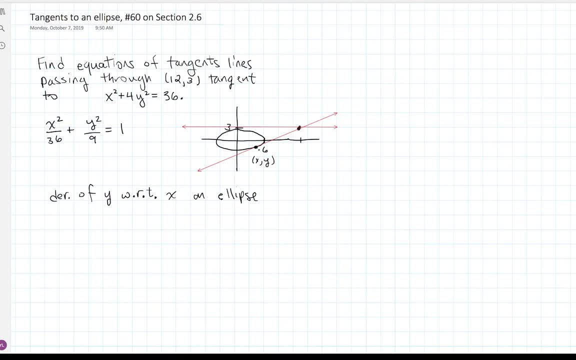 Since the derivative gives the slope of the tangent line to the curve, that should be equal to. well, the slope of that tangent line, which should coincide with the result of computing the rise over, run in between this point 12, 3 and the point the mystery, point X, Y. So this should equal. 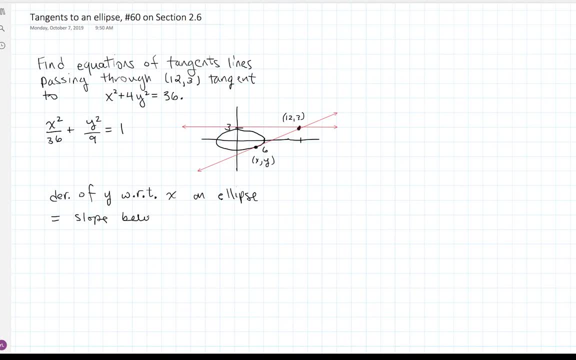 the slope sort of between X, Y and 12, 3.. So that's observation number one. Observation number two is that the point, the mystery point, lies on the ellipse. Okay, so I mean, this equation right here says that the X and Y coordinate of this point are related by 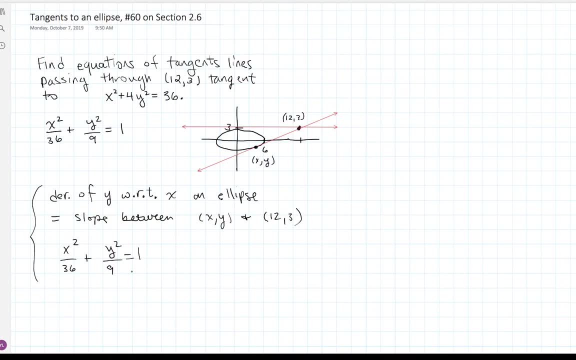 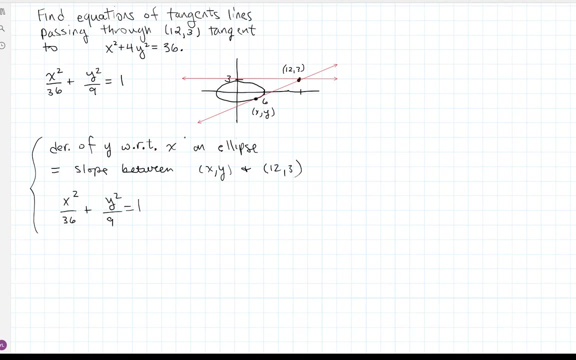 this equation. So it's, it's another piece of just algebraic information about the mystery point that'll become useful in solving the problem. Okay, so let me go ahead and translate the first observation into math from words. So, in order to compute the derivative of Y with respect to X, I'm going to want to use: 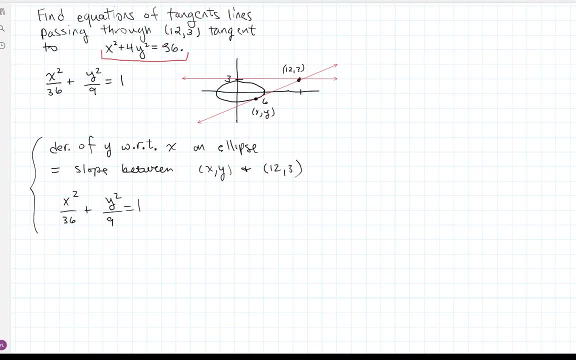 implicit differentiation to get dy dx, And I'll just go to this original equation to do that. So I'll perform a derivative with respect to X on both sides And keep in mind how you're evaluating your implicit derivatives. A first step is not. 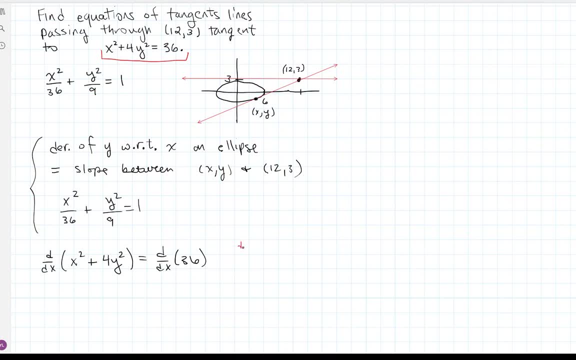 to write dy dx equals something. alright, If you're given a function explicitly, then you know sort of writing. the answer for the derivative can start like this: dy, dx equals, or f- prime of X equals, Y prime equals. But that sort of doesn't come until later when 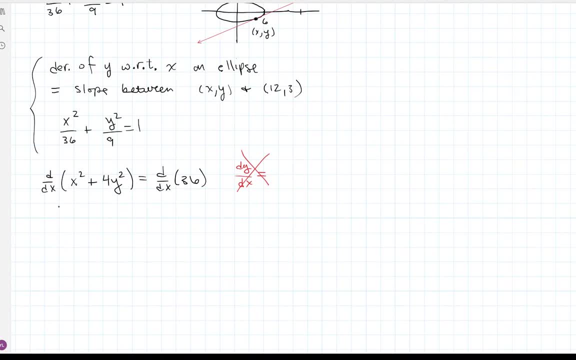 you're doing an implicit derivative, Okay, Okay, Okay, Okay, Okay, out as part of this computation. Okay, so I am using the method of implicit differentiation. Anytime I encounter a Y term, I'm interpreting Y as a function of X, and so I'm, in many instances, applying the chain rule. Okay, so I interpreted Y. 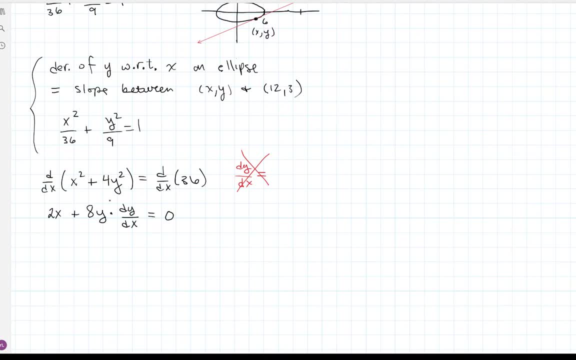 as a function of X. here It was being squared, so I applied chain rule Derivative of the outside using power rule. leave the inside alone times the derivative of the inside, which is dy dx. Okay, this allows me to solve for dy dx. so I get, I guess, minus 2x over 8y. so this is negative x over 4y. and now we 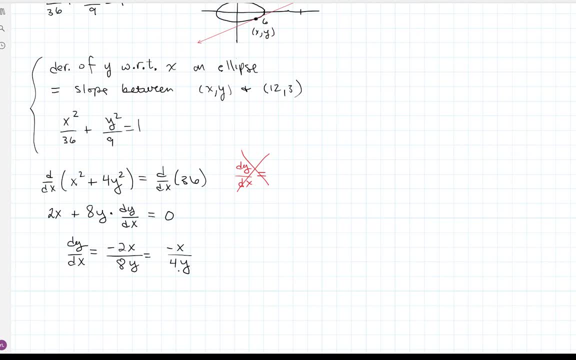 have this like typical implicit derivative, which is a you know formula that can be used to crank out slopes of tangent lines at any point on the ellipse. Notice how it depends on X and Y. Alright, so that was part one. Well, almost we have the observation one filled out. 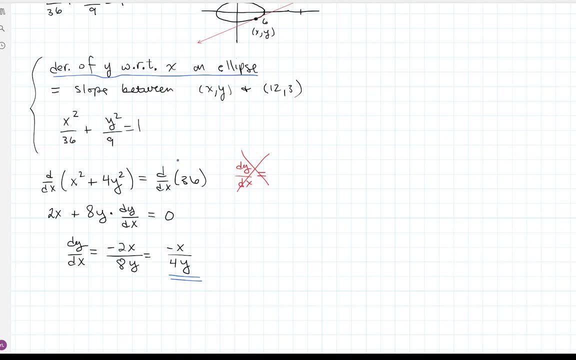 I've got the derivative with you know, of Y with respect to X for any point on the ellipse. Now the other part, slope between X, Y and 12, 3, is just your delta Y over delta X slope computation. So let me put that off to the side and then we'll set. 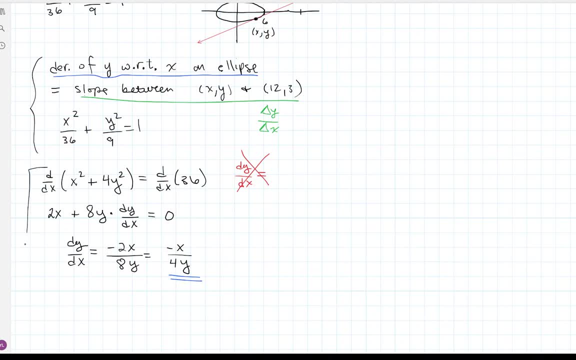 up. So this is the derivative, and over here I'll put the just the slope between X, Y and 12, 3.. So rise over, run. Now I can set up an equation, because I observed on the picture that that slope should be equal to the derivative. at that mystery. 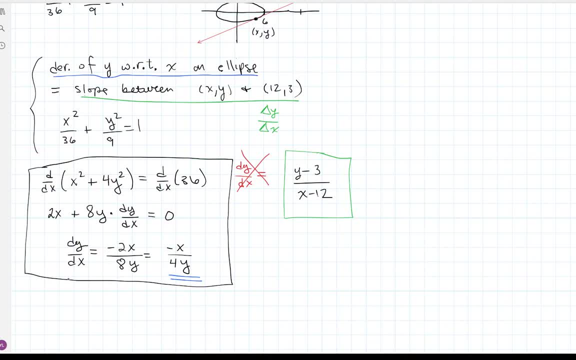 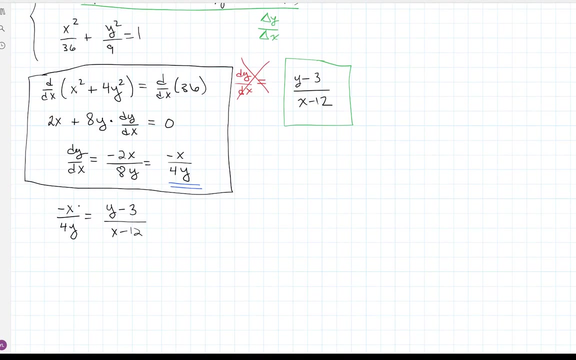 point. So I get my first equation from this negative: x over 4y equals y minus 3 over X minus 12. and then, as observed before, i'm going to pair this with the other information I have about the mystery point, which is that it lies on the ellipse, I think I. 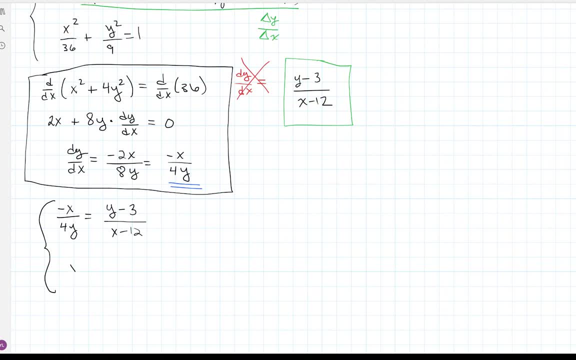 might write it on in the original form and you'll actually see why in a minute, in a sec. okay, so the point lies on the ellipse. so this is two equations right in two unknowns, and so if I just, you know, solve these simultaneously, hopefully I can get a value. 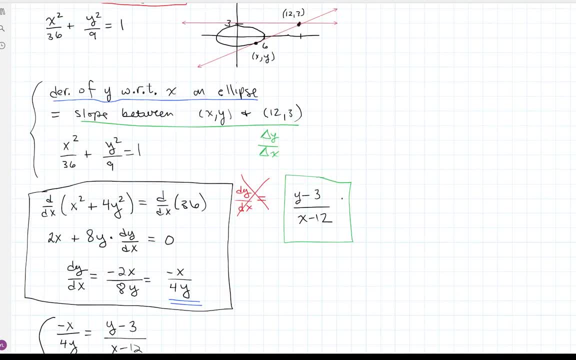 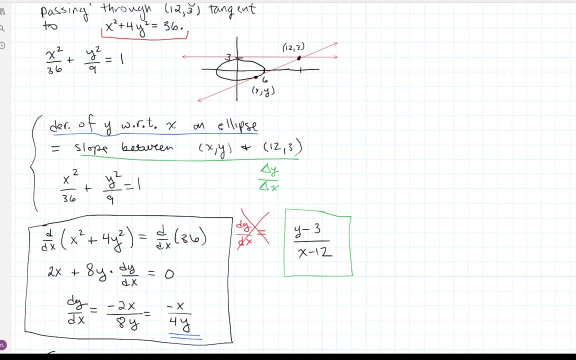 for X and a value for Y, and I should expect to get sort of more than one answer, because this system is good enough to detect any point. that sort of satisfies these two observations, namely that the tangent, that the point is a point of tangency and lies on the ellipse. okay, 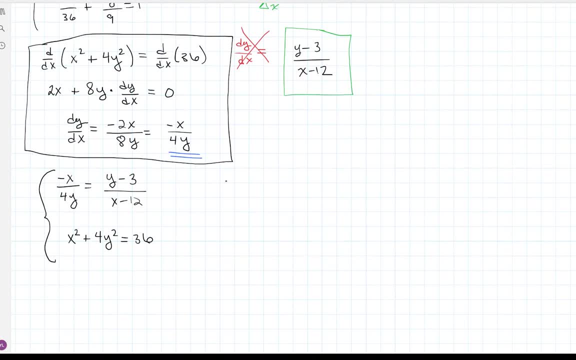 so let me just proceed with the algebra. I'm going to go ahead and get rid of the fractions over here, so I'll multiply both sides by X minus 12 and multiply both sides by 4y, and that leaves me with- let's see here- negative x squared plus 12x on the left and 4y squared minus. 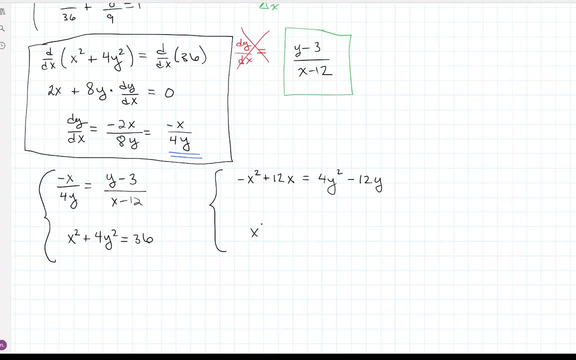 this 12y And then I'm not going to do anything to the second equation. just yet I do notice that if I bring the negative x squared over to the right, so I add x squared to both sides, and then I also move the negative 12y over to the left, a familiar expression appears: Watch. 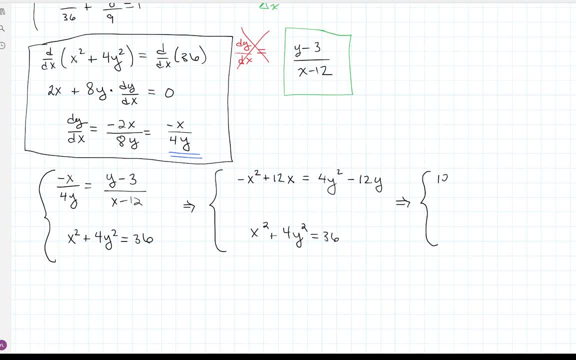 So I'm going to manipulate the first equation just as I said. So I'll have a 12y plus 12x on the left, and then on the right I'm going to have 4, I'm having some technical difficulties here. Okay, I'll have 4y squared plus x squared. 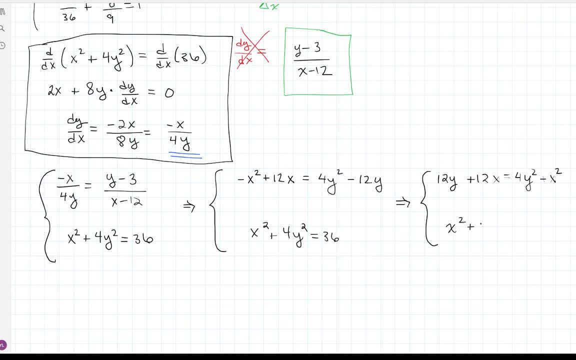 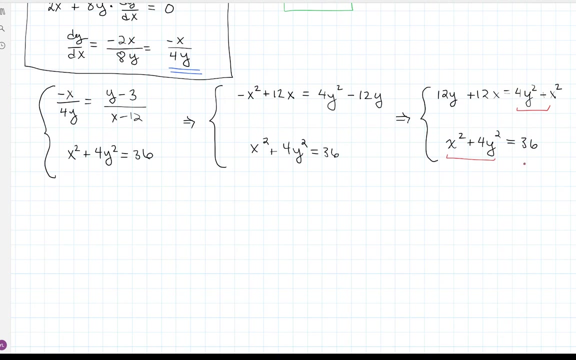 And 4y squared plus x squared is exactly what I have on the left-hand side of the second equation. So I'm going to have 4y squared plus x squared. So, with that observation that this expression is the same as this expression, this allows: 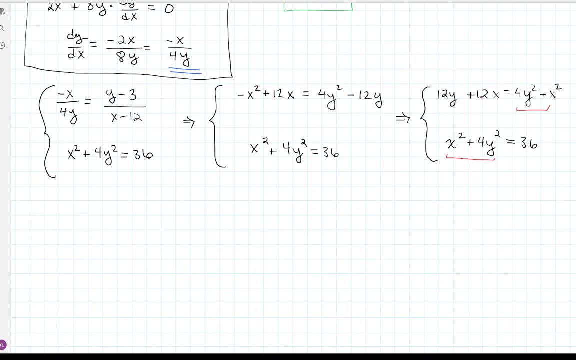 me to deduce that 12y plus 12x is actually equal to 36.. So I'm imagining coming down here and replacing this expression with what it's equal to. So I get that this gives me: 12y plus 12x is 36,. let me clean this up a bit. I'll just 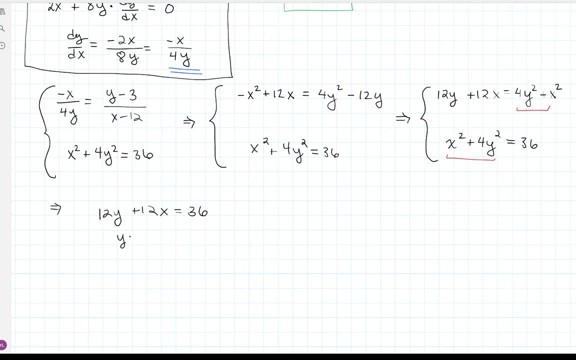 divide through by a 12, and maybe I'll move the x to the other side so that'll give me y equals 3 minus x. Okay, I didn't quite. I mean if you're lucky when you sort of make your first algebraic. 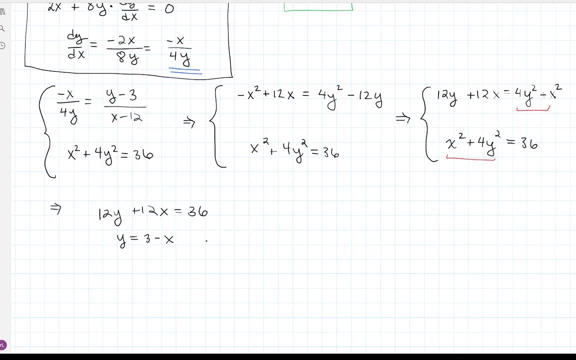 observation of how to combine your equations, you might get one of the unknowns completely solved, for I don't have that just yet, but I think I can take this back to maybe the second equation again and reduce it to a one variable equation. 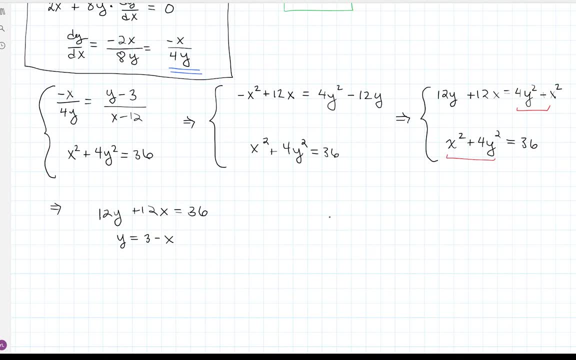 So, like I have y in terms of x now, So So I could use either of the equations to swap out a y in terms of x. So that's what I'll do right now, I'm just going to go ahead and take the y equals 3. 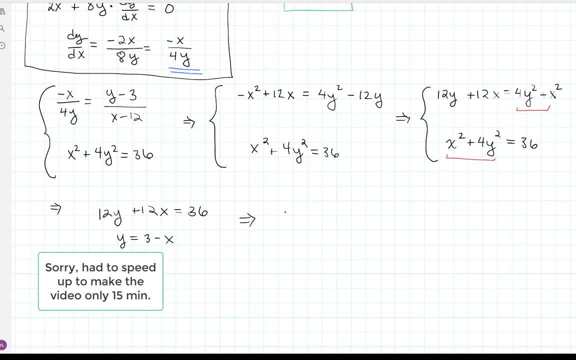 minus x and swap it out in this equation here. So that leaves me with x squared plus 4, 3 minus x squared equals 36.. This is now a quadratic in x, so I'm just going to put it into a good form and try and 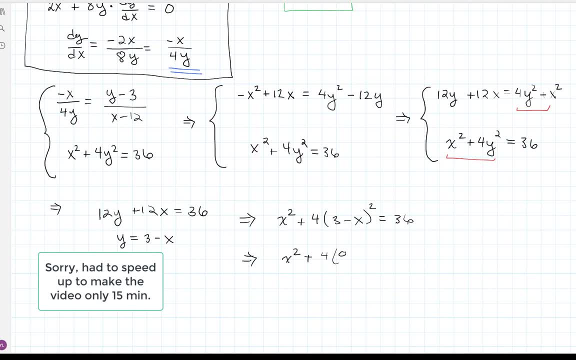 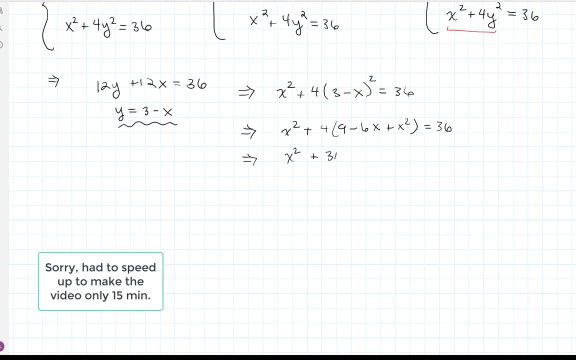 figure out what the solutions are. Alright, so we've got 9 minus 6x plus x squared. So okay, multiplying things out, I'm going to have x squared. I've got 36 minus 24x plus 4x squared. subtracting 36 from each side and gathering like terms, I guess I've got. 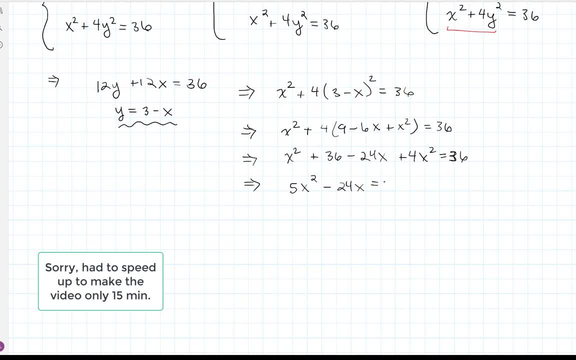 5x squared minus 24x equals 0.. And this means that, oops, factoring out an x. I see two solutions for x: the x coordinate of the point of tangency, And this is kind of what I expected right. 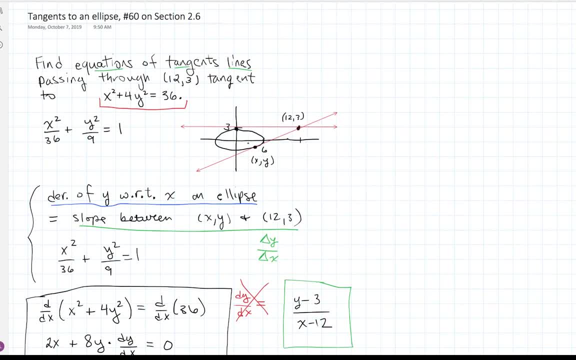 I've got x equals 0. I knew about that x coordinate all along. That's the x coordinate of this point: 0, 3.. And the other one: I expected x to be some like positive number less than 6.. 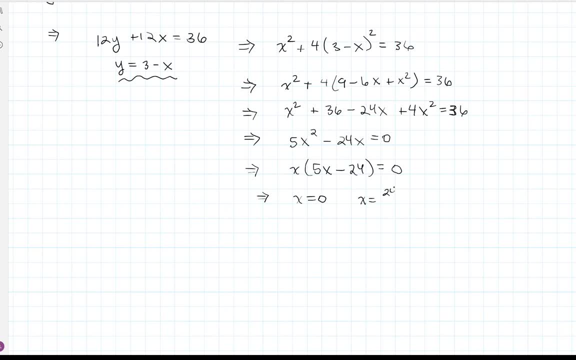 So I mean, what I have right here is 24 divided by 5, yeah, that's even a little bit less than 5.. So let me go ahead and take these two, like the x coordinates of these two points of tangency. 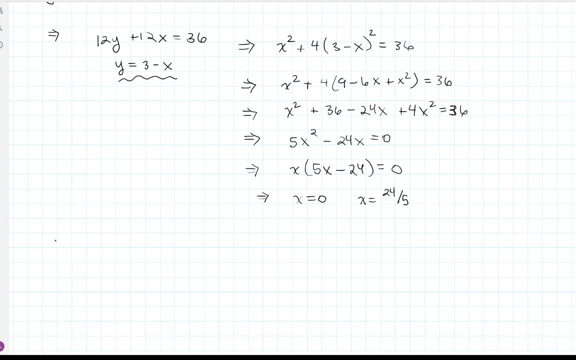 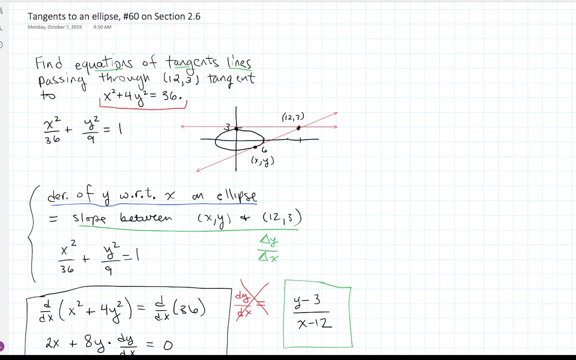 and figure out what the corresponding y coordinates are. so I'll have these two points completely. The question is about equations of tangent lines, so I'm going to need to take that information and then information about slope to build the equation of the tangent line, just as usual. 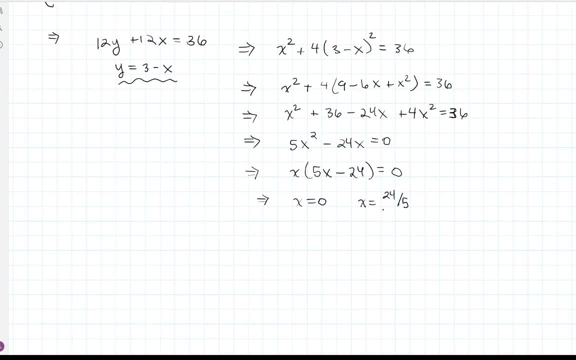 okay. So in order to figure out the y coordinates of the points of tangency, I'm just going to use this observation up here that the y coordinate is 3 minus x squared. So I'm just going to use this observation up here that the y coordinate is 3 minus the. 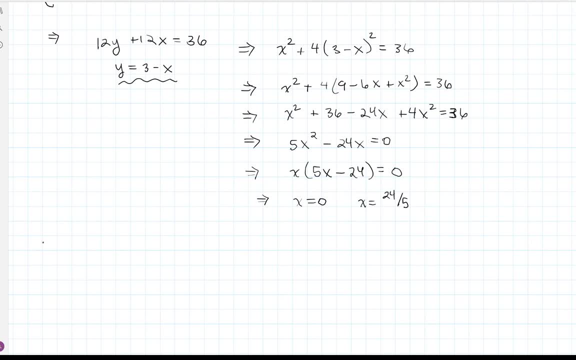 x coordinate. So let's obviously just do that with a 24 over 5.. If I have x is 24 over 5, then y is 3, minus that 3 is 15 over 5, so I've got 15 minus. 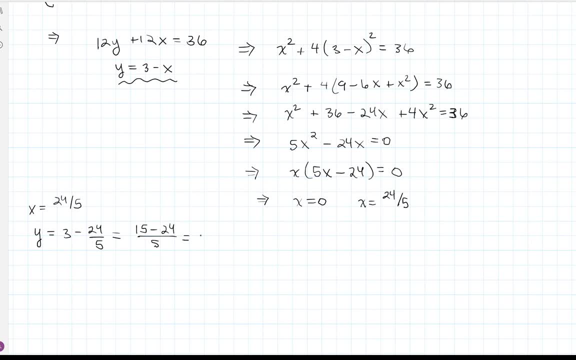 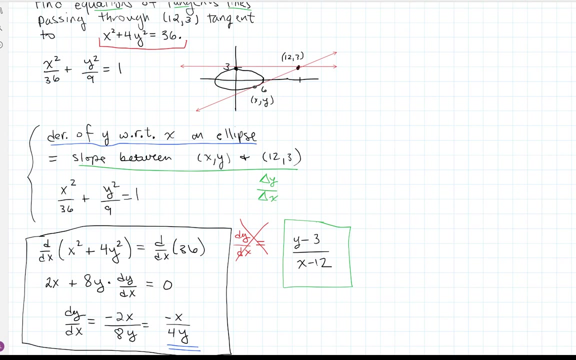 24 over 5, and that is like negative 9 over 5.. This is a negative y coordinate. this isn't a surprise as well, because if you look up here, the y coordinate of this point is definitely below the x axis, right. 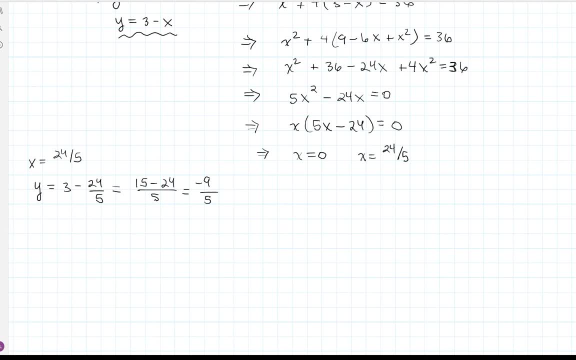 So the fact that it's negative is reasonable. It's also like less than negative 2, which is also, I guess, pretty reasonable. I don't mean less than I mean in magnitude. it's less than 2 below the x axis, which means 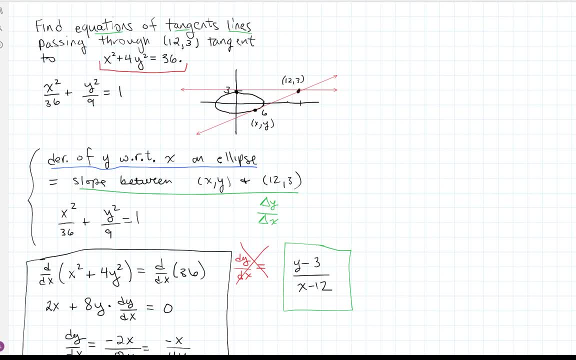 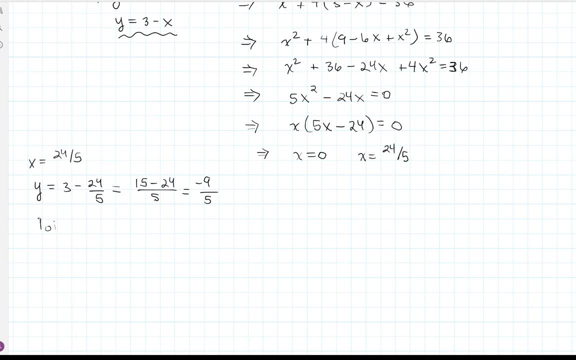 it's not like extending past the bottom of this ellipse, so it's a reasonable number. I say Okay. So I know the points of tangency completely. now The points of tangency, two of them. tangency pen is crapping out, I'm not sure why. 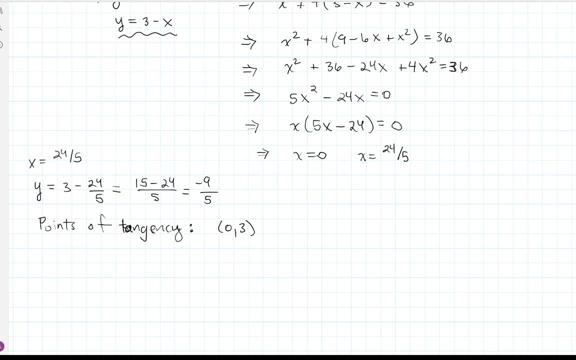 I knew about 0, 3 in the beginning, and now I've just reinforced that. and then the new one that I found is 24 over 5, negative 9 over 5.. So now I'm ready to report the two tangencies. 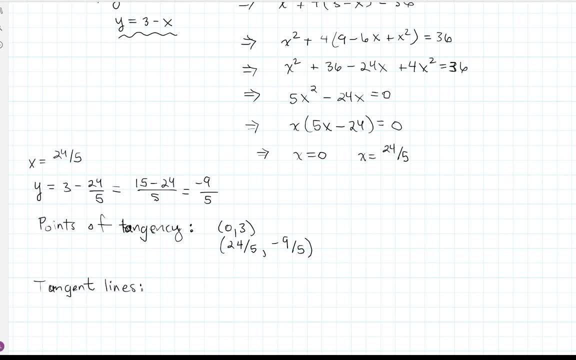 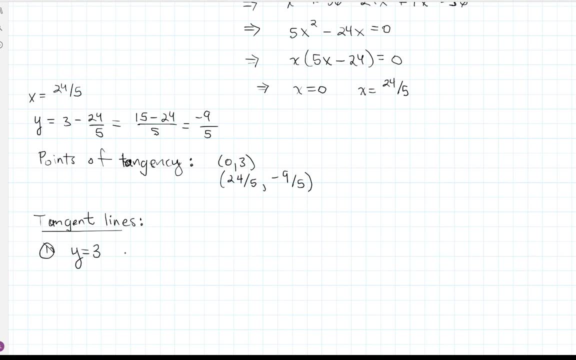 Okay, Line number one is a horizontal line at y equals 3.. That is the answer again I knew about from the beginning. The second tangent line goes through this point and has some slope right. I can glance up at my work here. 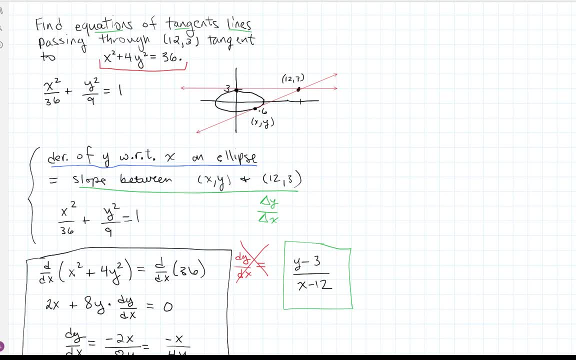 I can just remember where this all started, you know. now I know the coordinates of this point. The slope of the tangent line is the slope between those two points. so I'm just going to do, you know, a rise over run computation here.